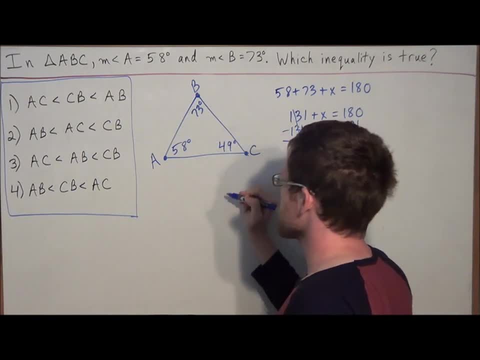 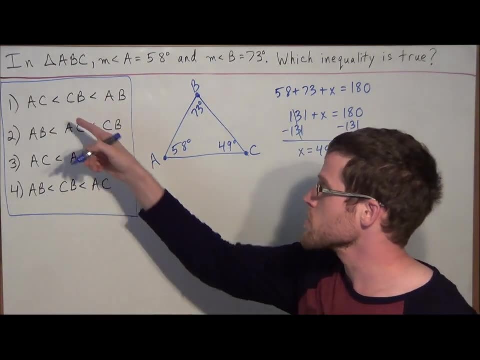 So this is an important step: finding the three, the measure of the three angles of the triangle. But next we look to our answer choices and notice that all of the inequality signs are less than So. this is telling us- this is just a helpful trick- that when you 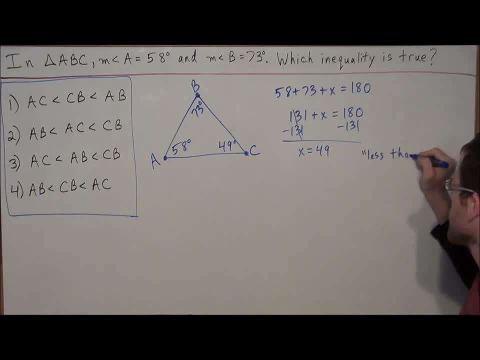 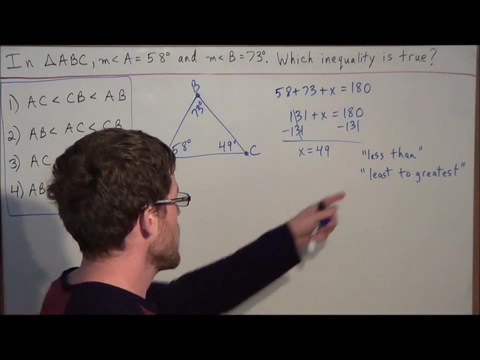 read less than that. they ordered the sides from least to greatest. So the key is to say the inequality out loud and since it's a less than sign for all the answer choices, less than should prompt you to think in terms of least to greatest. So next we're going. 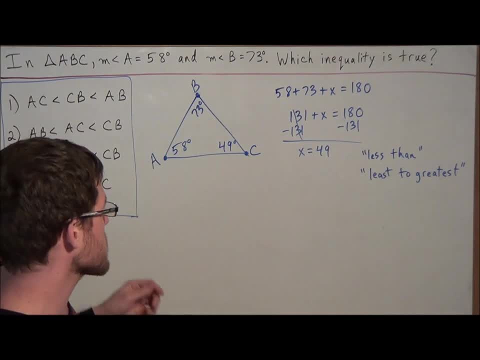 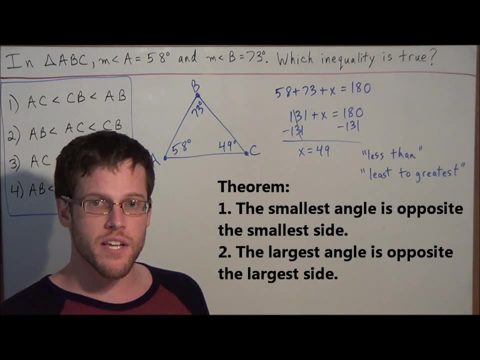 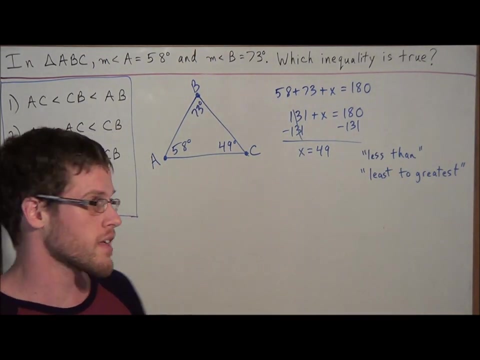 to use the theorem, our theorem, which states that the smallest angle in a triangle is opposite the smallest side. Or the other way we could say it is that the greatest angle is opposite the greatest side. But because we're going from least to greatest, we want to start with the idea that the smallest 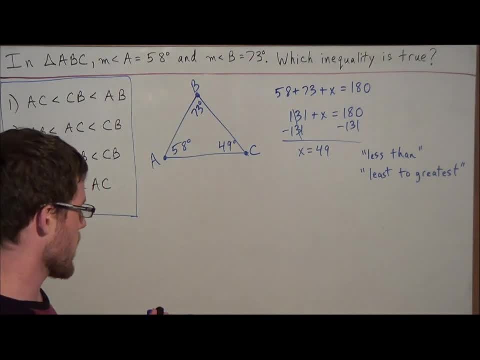 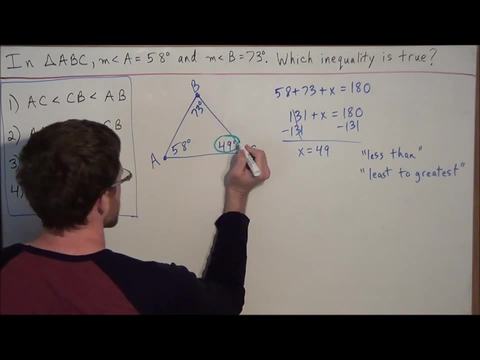 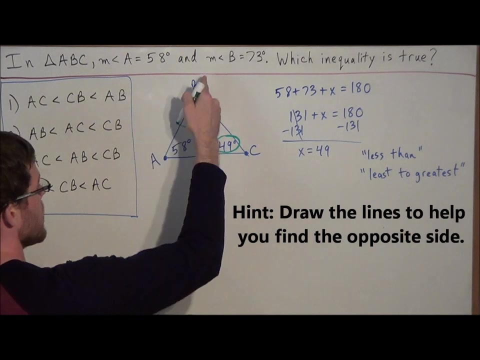 angle is opposite the smallest side. So that means we have to start with the smallest angle in our diagram And notice that 49 degrees is the smallest angle. So we go opposite of angle C And notice, when we go opposite of angle C, the first side we hit is side AB. 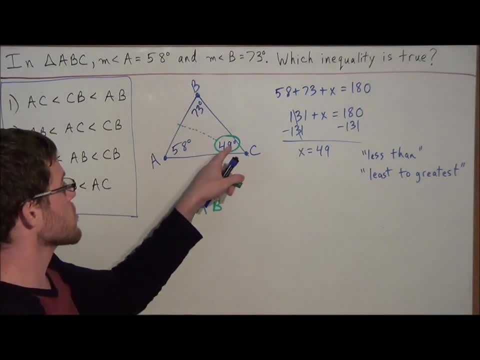 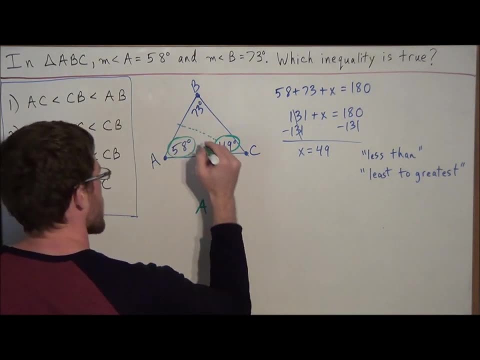 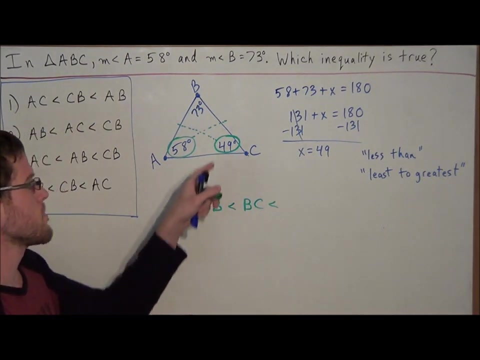 So AB is going to be the smallest side in our triangle. So after 49,, the next smallest number is 58. So this tells us that the next smallest side is going to be side BC. And now, by process of elimination, we know the last side is AC. 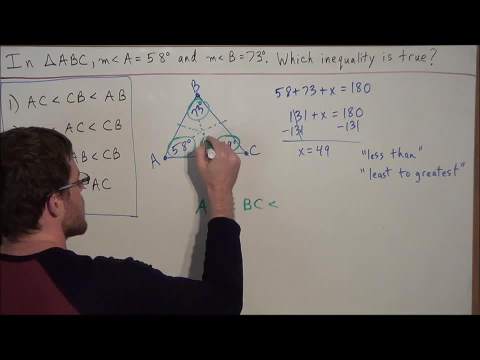 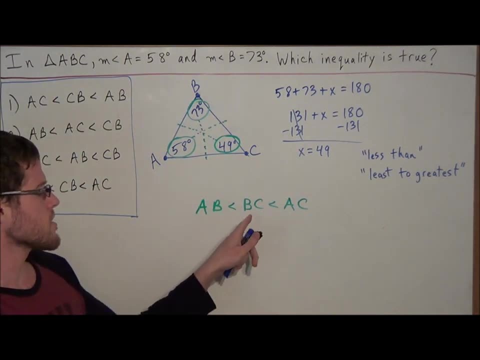 Or we could go to the biggest angle, 73. We go opposite to side AC, which tells us that the order of the sides is that AB is less than BC, which is less than AC. So we go to our answer choices And notice that choice four matches what we just found. 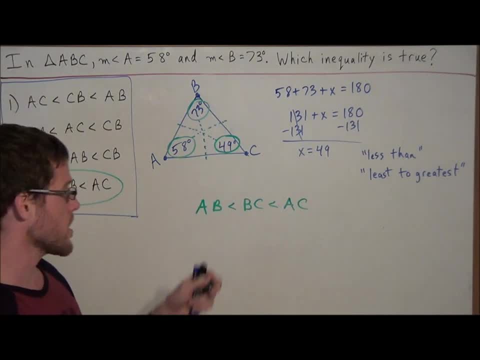 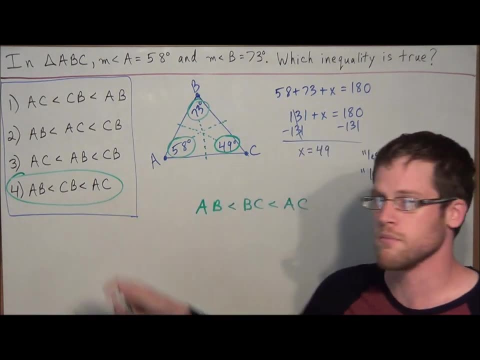 One small little detail: BC and CB are the same size, So that when you do this on your own, you have to be able to reverse the letters in the event that they are flipped, as it was with CB here. OK, well, this is going to conclude this video. 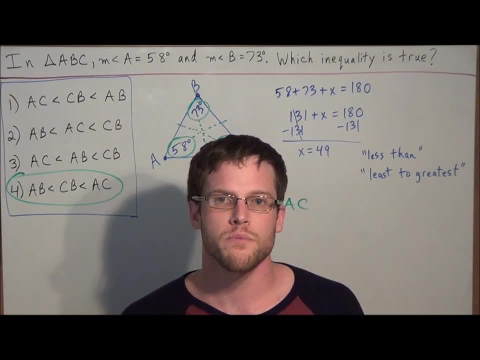 on angle-side relationships in a triangle. Thank you all for watching And I hope that this was helpful.